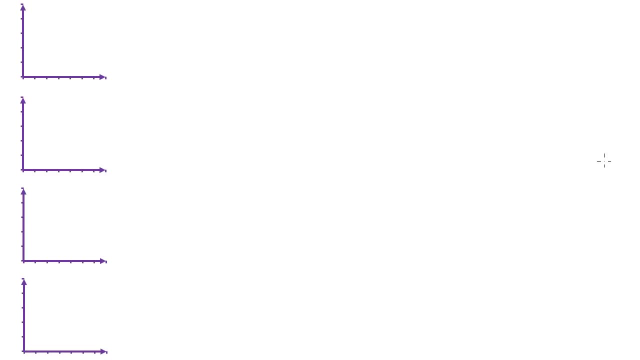 is Pearson's product moment correlation coefficient- Don't say that five times fast. So when we had a scatter plot where the dots fell in a perfect straight line, something like that, we said that was a perfect relationship. And then the next level of strength down from being a perfect relationship was for 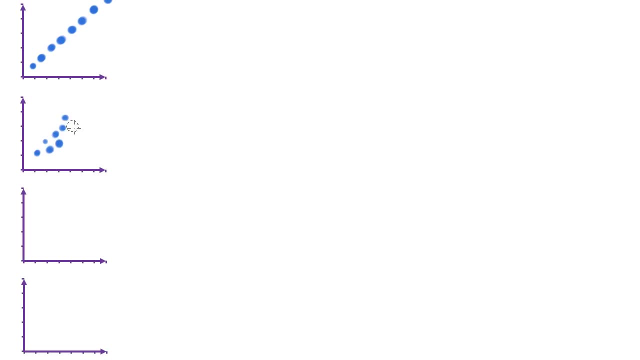 them to be pretty close to being in a perfect line, but just not quite, And that we called a really strong relationship. And then they got a little bit more higgledy-piggledy, They got a little bit more spread out and we called this a moderate relationship. The strength: 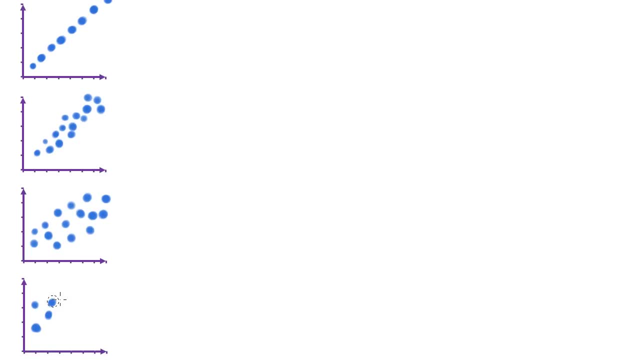 was kind of moderate, And then they spread out even more and they looked even less like they were in a line, although they still did follow a linear sort of line, And then we called this a fairly weak relationship. Now the r value is a way of describing that relationship with a number. We give it a statistical 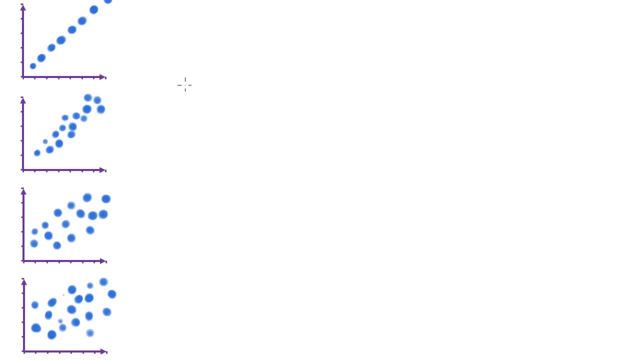 number, this Pearson's product moment correlation coefficient number, so that we can compare things rather than saying weak or strong. That's a bit vague. So a perfect relationship like this, where everything falls perfectly in a line, that's an r value of one. 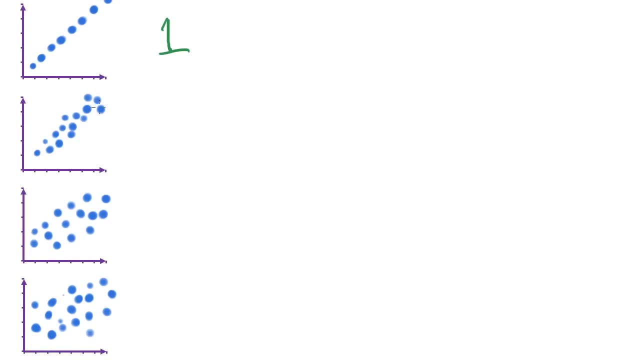 When you have a strong relationship like this one here, where things are quite, they follow the trend really nicely, we would give that an r value of 0.75 to one, somewhere between 0.75 and one. So, for example, 0.8,, that's a really strong relationship, or 0.9, something. 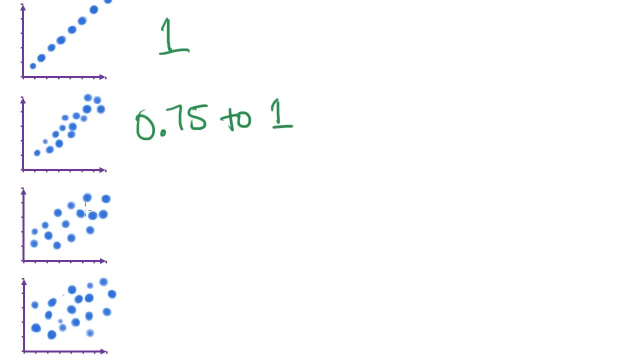 like that Moving along. when you had a moderate relationship, that would be somewhere between 0.5 and 1.5.. When you had a moderate relationship, that would be somewhere between 0.5 and 1.5, and 0.75. the weak relationship down here is going to be between 0.25 and 0.5. so 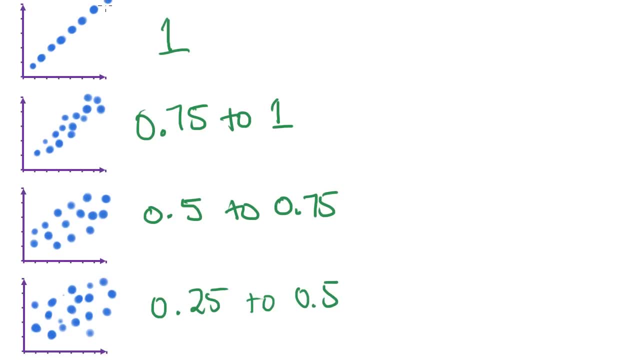 one is perfect, all in a line. 0.75 to one is very, very strong. 0.5 to 0.75, moderate, 0.25 to 0.5 is weak and anything less than 0.25. there's not much of a relationship at all. you'd say almost no correlation. they, hardly they. 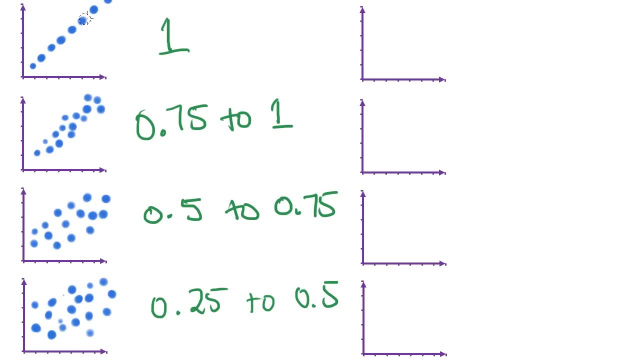 hardly relate. now, if you notice, all those relationships that I've drawn on the right there go in a positive direction. they go up the hill, like that. so what happens when we're talking about a negative relationship? so, for example, we have a perfect linear relationship, but they're going down the hill. they're 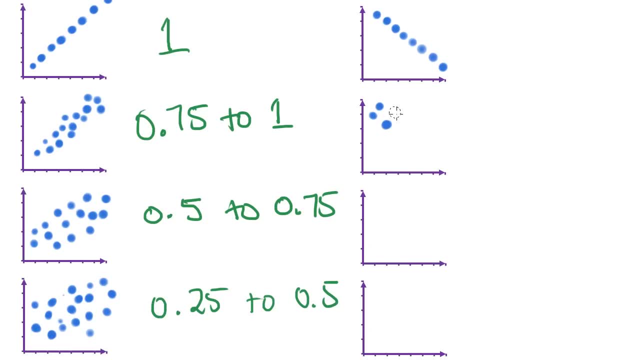 going in a negative direction. and again, a strong relationship, but it's a bit more on the negative side, or a moderate relationship, or a weak relationship, negative. well, the nifty thing here is the R value is just is the same for the positives. it's just negative. so a perfect relationship, that's a negative. 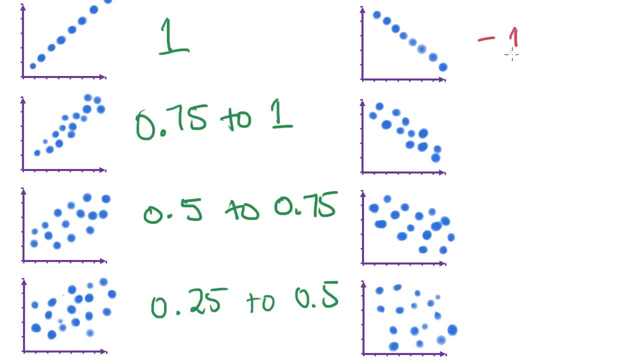 relationship has an R value of 0.75. negative 1. a strong relationship in a negative direction would have an R value somewhere between negative 0.75 and negative 1. a moderate, moderately strong relationship in a negative direction would be- can you guess, from negative 0.5. 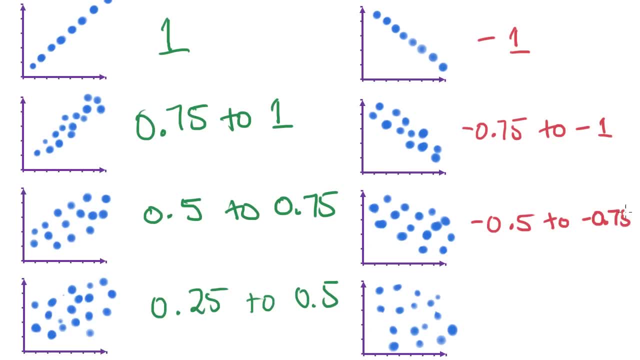 to negative 0.75 and of course, a weak relationship that just happens to go in a negative direction would be somewhere between negative 0.25 and negative 0.5. so a negative R value doesn't mean that there's a poor association. negative doesn't mean like 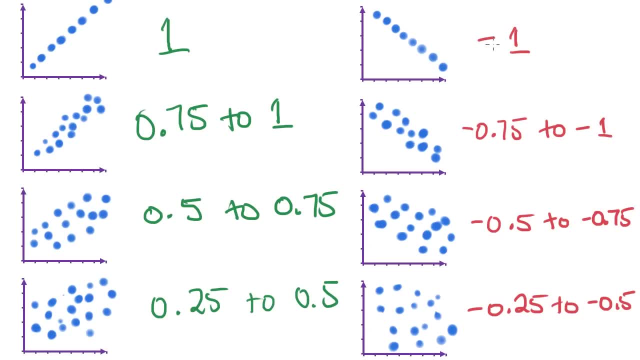 oh bad. you know, like that there's no association there, because negative 1 is a great R value, because it means it's a perfect relationship. so 1 and negative 1 for R values are both. you know what you're aiming for. they both tell you. 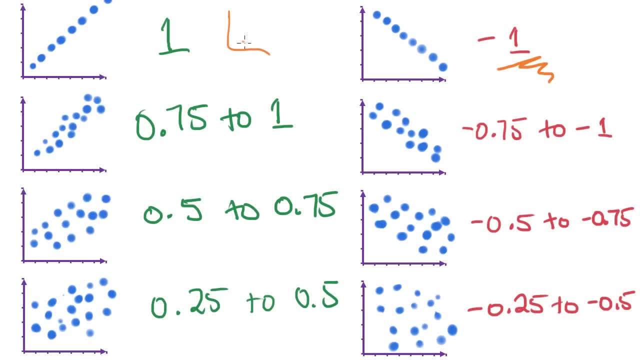 that there's a perfect relationship there. it's just that one of us tells us we're going up the hill and one of us tells us we're going down the hill. so as independent values increase, the dependent values increase as well, or as independent values increase, dependent values decrease. both are a perfect. 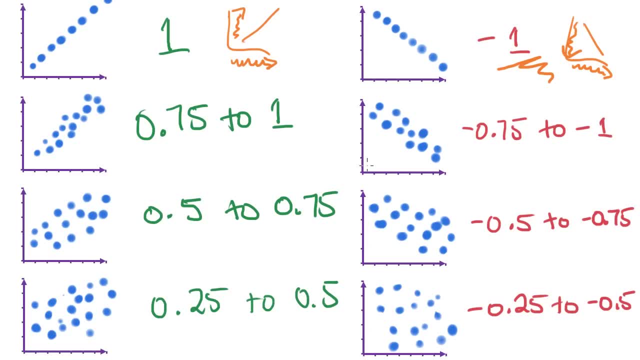 correlation. it's just that we get to find out which direction we're going in. so, as you can see, an R value is always going to be between negative one and positive 1. So an r-value can't be, for example, negative 3, or it can't be. 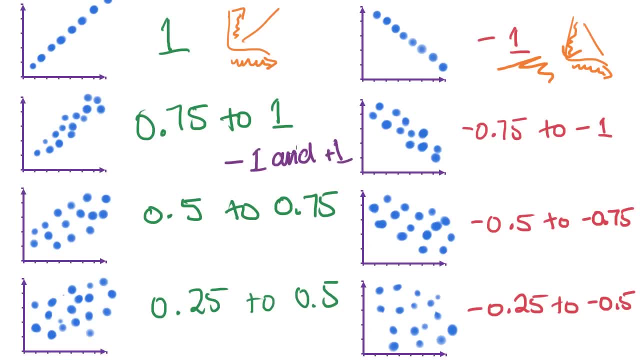 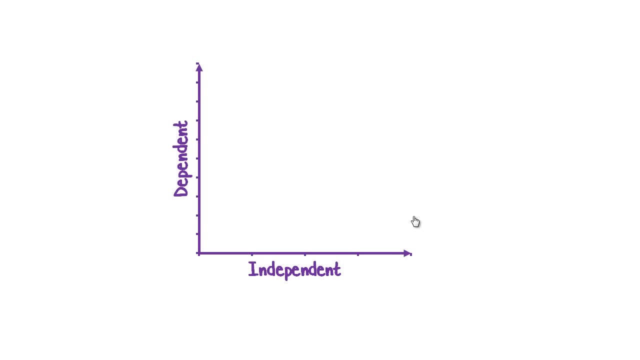 positive 2.759.. Your r-value always has to fall somewhere within this range. If you get another number, you've done it wrong. basically, So, if an r-value has to be somewhere between negative 1 and positive 1, what does an r-value of 0? 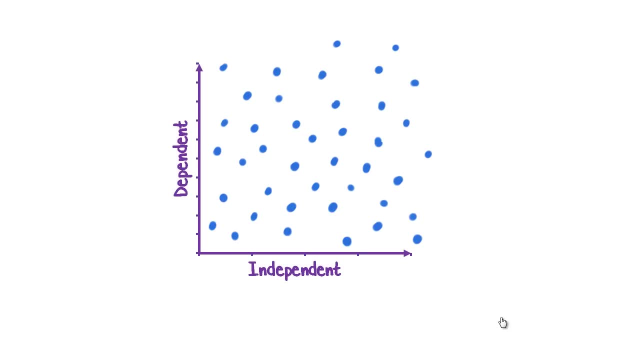 look like It's completely random When you scatter plot has no association. it looks like the independent variable and the dependent variable don't relate to each other. they don't have a relationship. you can't see any correlation going on there. they're just not having a party. then you have an. 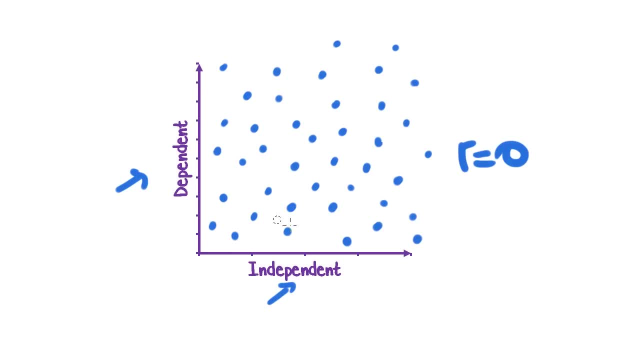 r-value of 0, because there's no strength to it whatsoever. It's neither one direction or the other, it's not in any way strong, it's not even weak, it's just nothing. So r is 0.. Now here's a couple of things to watch out for. Firstly, this works for linear. 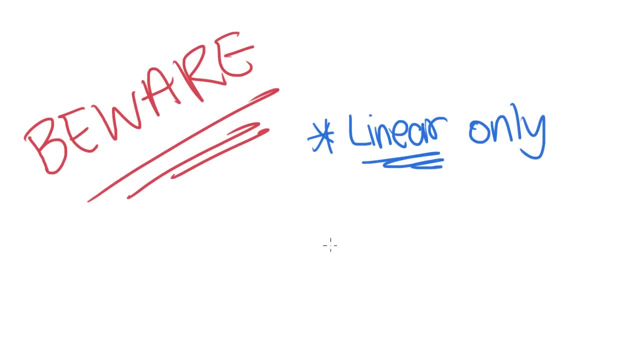 relationships only. If you get a scatter plot that has dots looking something like this- pardon my terrible drawing but say it has a roughly curvy sort of shape to it- then don't apply an r-value. That's not going to work. 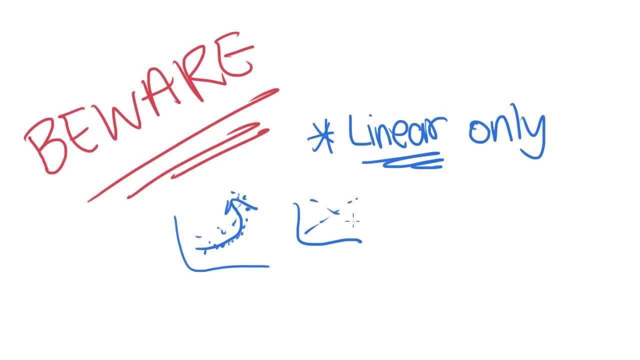 Pearson designed it for these straight line graphs, either that way or that way. So linear relationships only. And the other thing to watch out for is outliers. Outliers, those hinky little buggers, will screw this up. If you have a scatter plot that looks like this, it's perfect, perfect. 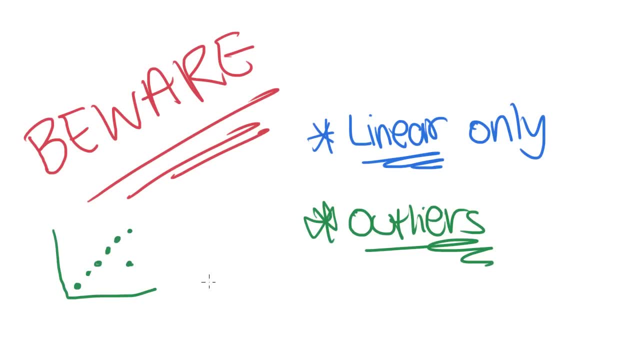 perfect, perfect, except it's got a dot out here. then your r-value might be something like 0.6, which really doesn't tell you that, hey, this whole thing is a perfect relationship, except for one little freak of the measurement out here. So outliers screw up this value. So you need to be. 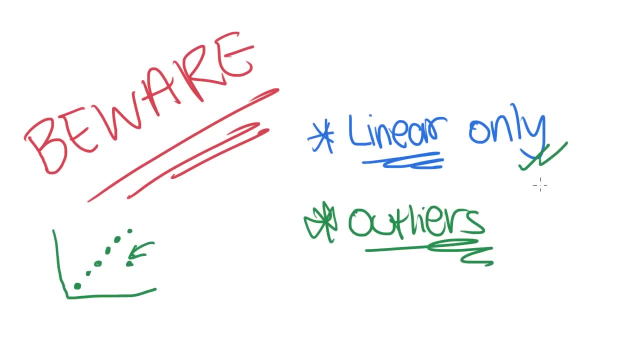 really careful that you're definitely using linear, you're definitely talking about a linear relationship and there are no outliers before you apply this. So what I would say is: draw yourself a scatter plot first. If you've got an r- value question, draw yourself a little scatter plot either on your calculator. 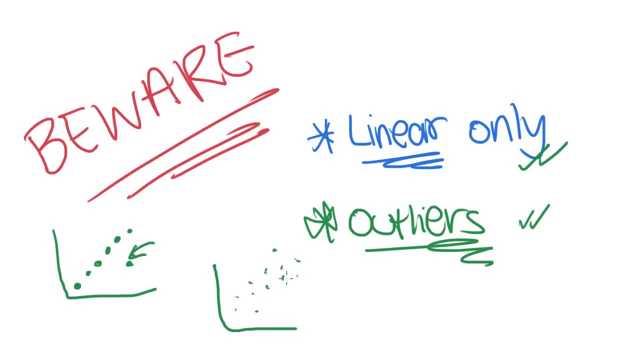 or quickly by hand, and you can check a couple of things. Firstly, you can check if it has a linear relationship, then you can check if there are any outliers, and then you've actually got a pretty good idea from your scatter plot of what your r-value should be. For example, if I put 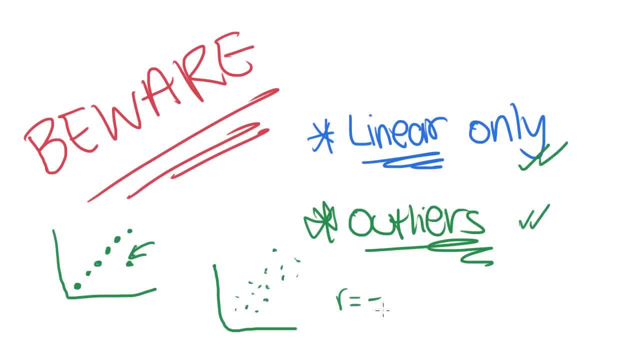 this into my calculator and I got an r-value of negative 0.5, for example. I go hang on a second. I must have done something wrong either when I plotted it or when I worked out what the r-value was, because this should be a positive r-value. 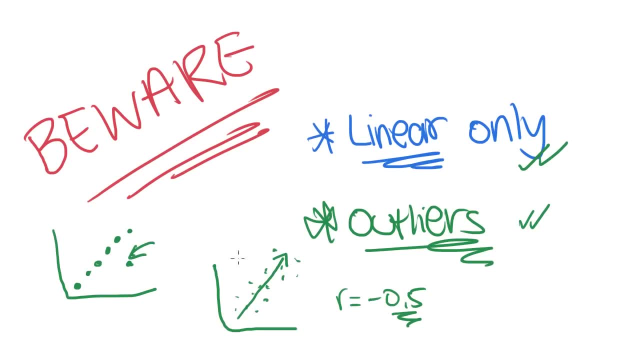 So if I get a negative one, I know I've done something wrong. So draw yourself a little scatter plot first, and then you can check off these two things and you can also give yourself a nice little guesstimate of what the r-value should be roughly Okay. so how do you work out the r-value? 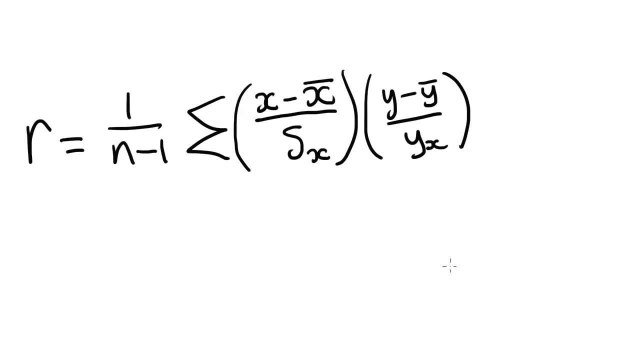 There is a formula and it looks like this. but here is the good news: In further maths, you don't have to worry about this. You don't have to do this manually. You never have to work this out. You can always use your calculator. So finding 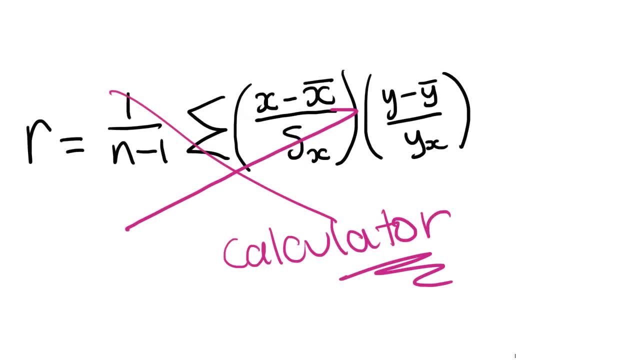 the r-value on your calculator is different depending on which one you have. Most of you will have a CAS, in which case you go to the lists and spreadsheet page and then you press menu statistics, stat calculations, and then three for linear regression, mx plus b, and then you put in your variables and 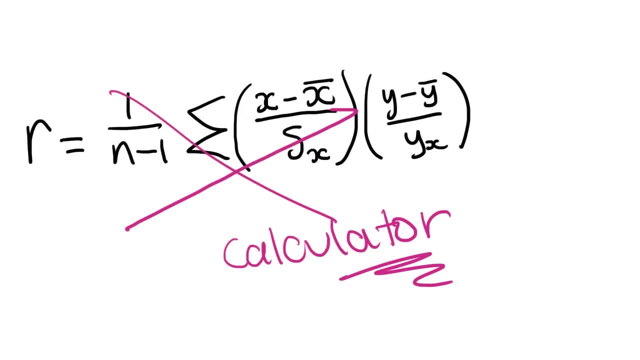 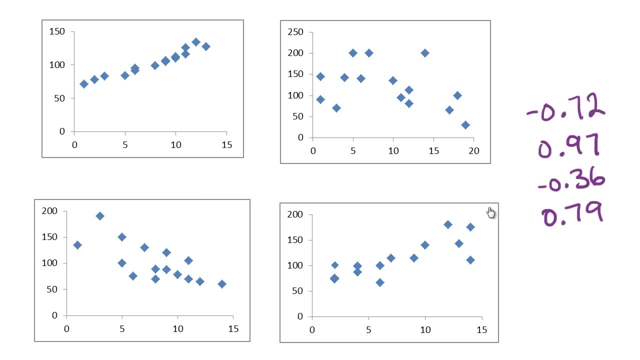 you hit enter okay, and you scroll down the little list of things it gives. you will give you m, b, r, squared and r, and then you just read it off. So now to practice that. here are four scatter plots that I've just quickly drawn, and: 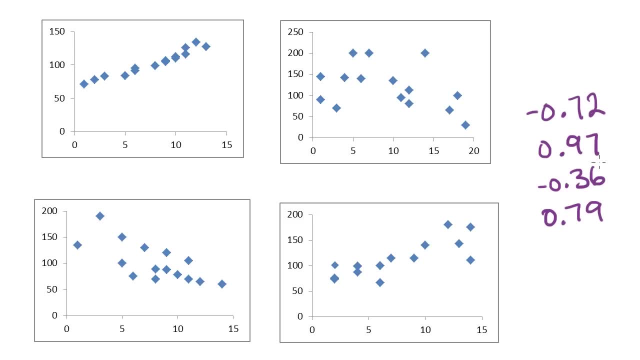 these each have an r-value of one of the following four. So we've got negative point seven, two, positive point nine, seven, negative point three, six and positive point seven, nine, and so hit pause and see if you can work, work out which of these four corresponds to which of these r-values. Okay, let's. 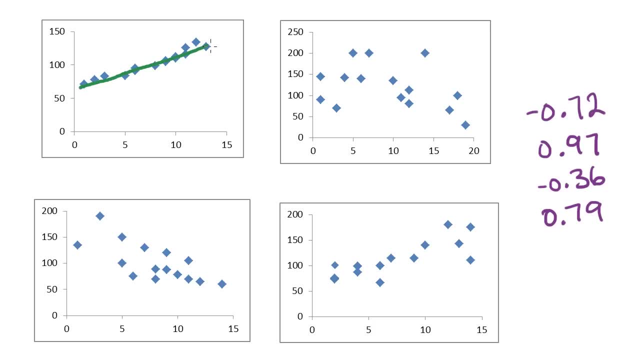 start with this first one here. This looks like it's going in a positive linear direction up the hill that way and it's fairly close to being in a straight line. These dots all fall really well on that line. It's very, very strong. so the r-value is going to be close to positive one. so 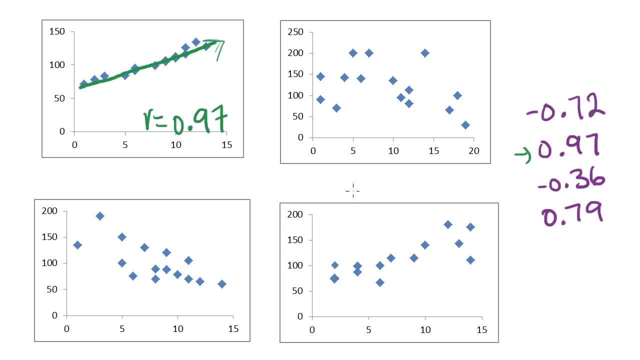 this one here looks good, so it's r of 0.97.. What about this one here? This one's not got a very strong correlation. The relationship doesn't really fall that well in a line. It does kind of have this shape that goes down this way, though. so 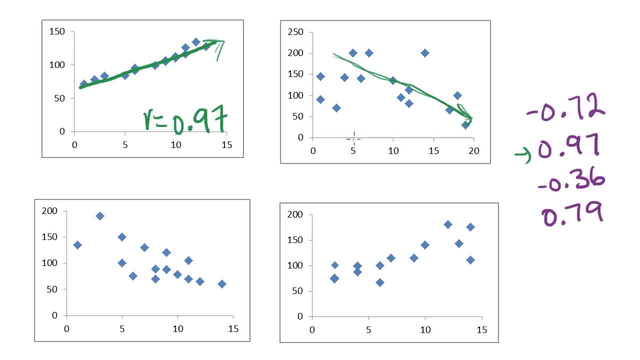 if it was going to be linear, it'd be negative going down there. So the r-value for this one is going to be negative and it's going to be closer to zero than negative one, because it's not very strong. So it's likely to be this one, negative 0.36.. What about this? 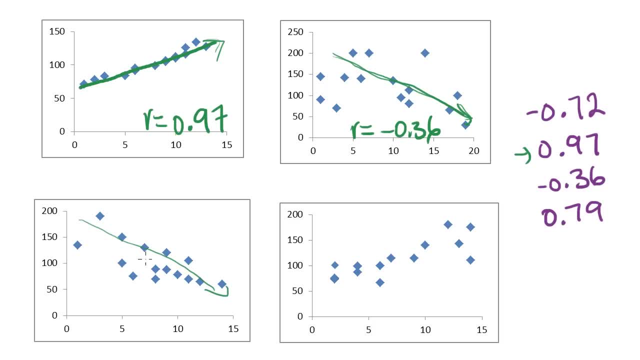 one over here. Again, we've got this sort of negative direction going down there, but this one's much closer to falling into a line than these ones were. So this has got a stronger relationship. it's going to be closer to negative one. So that's this one here. negative 0.72.. And finally, what about this one? This is: 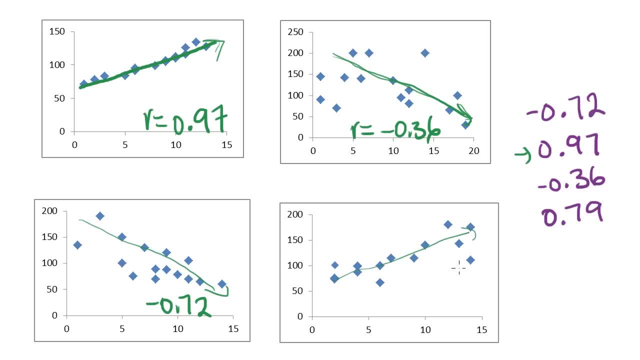 going in a positive direction, so it's going to be positive number, but it's not as close to falling in a perfect line as these ones were. It's still pretty strong though, so it's probably going to be above 0.75. and what do you know? our last option is 0.79 positive. 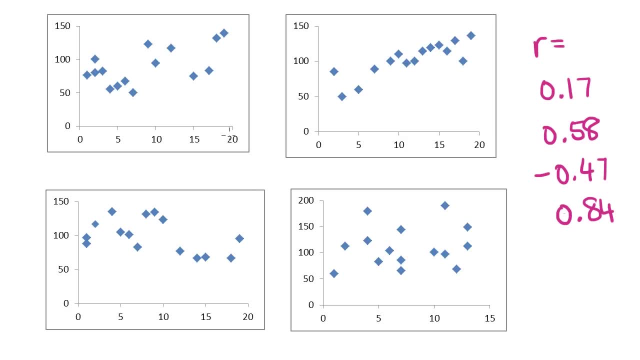 So same exercise again, new scatter plots. so here are four scatter plots and four r values. see if you can work out which graph corresponds to which r value. So this first one: here it's got a sort of going up the hill shape. it's got a generally positive.